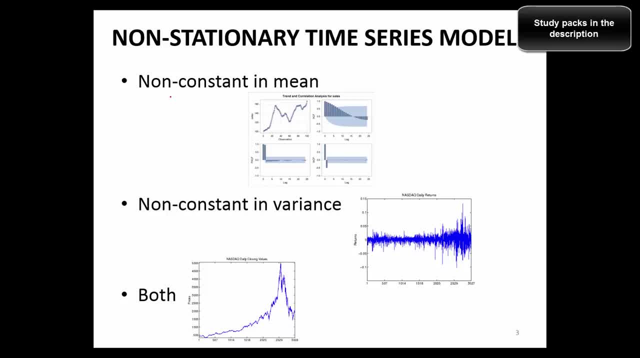 what we mean by stationarity in time series data. So the two important things are mean of the time series and the other one is the variance, right? So we are concerned about the mean and variance of the time series when trying to understand whether the series is stationary or. 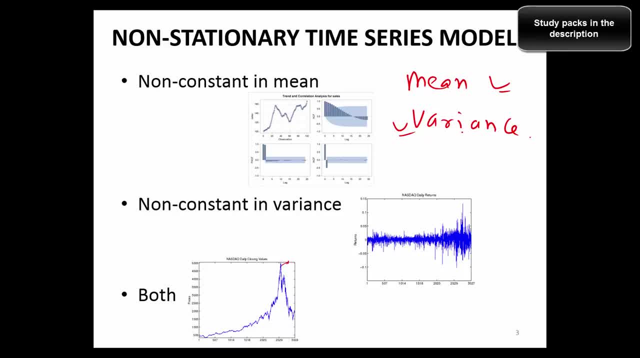 not. So mean and variance have to be constant for a time series to be called as a stationary time series. Sometimes the mean could be non-constant. The first case of non-stationarity could come from the mean being non-constant, As you can see in the particular, you know, time series graph. 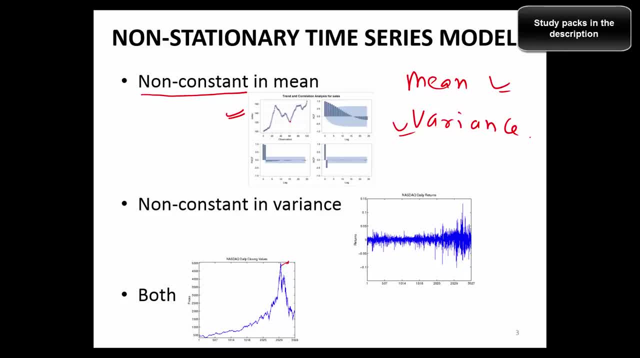 you can see, the mean is not constant in nature. It is increasing. right, It is an increasing trend. So the mean is increasing with time and that's a typical case of non-stationary time series. Sometimes the non-stationarity could come from. 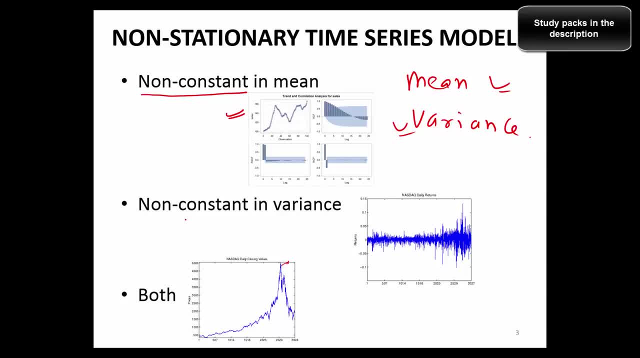 by it could be through variance as well. So we could have a non-constant variance and that could also be the reason for non-stationarity, And sometimes, it you know, there could be both non-constant mean and non-constant variance. So here is a typical example. So the second example is a case where 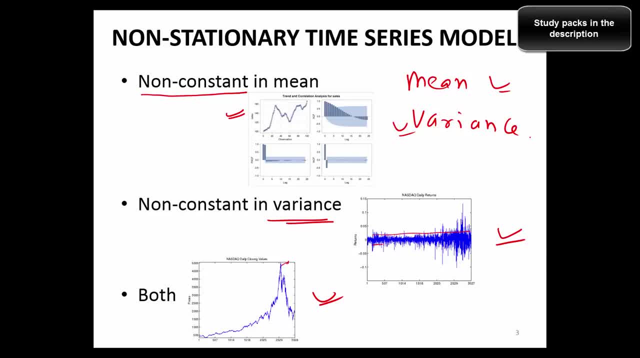 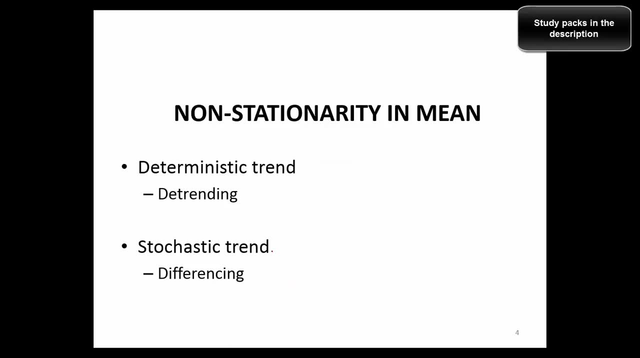 you know it's a constant mean. you can see The mean is very much constant, but you know the variance is actually. you know variance is actually increasing over time, right? So that's a typical case of non-stationarity due to non-constant invariance. okay, 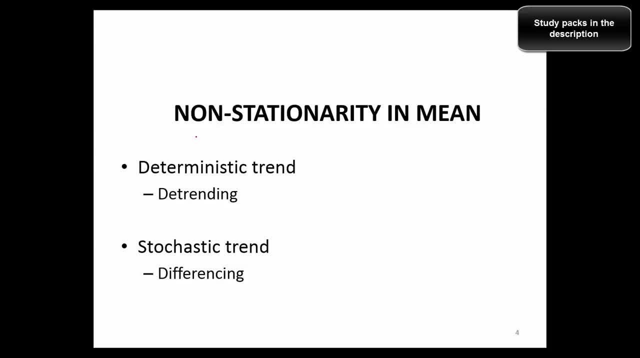 So in this particular session we will only be concerned about the non-stationarity in mean. okay, So we're not concerned about non-stationarity in variance, because that's where the focus is for this particular session. and unit root is something that we can relate to, a time series data where we 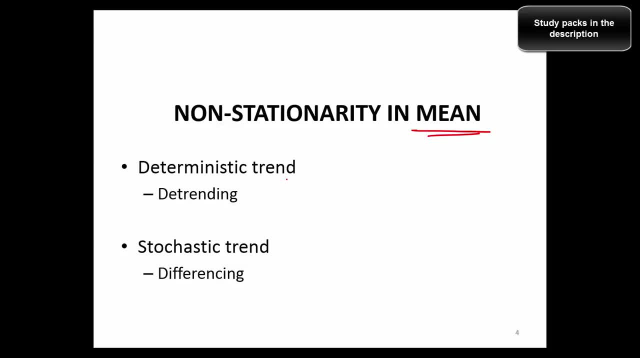 have non-stationarity in mean. There are two aspects to non-stationarity in mean. In one case, you will have a deterministic trend, and we'll talk about what deterministic trend is, and the other one is where you have a stochastic trend. okay, So deterministic, as you understand from the word. 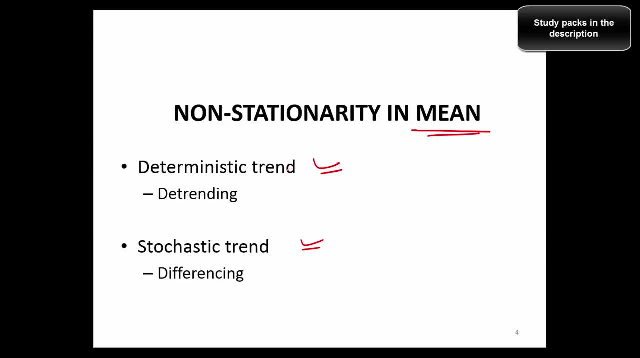 itself something that we can easily determine okay, So without having to go through more of a you know uncertainty, okay, Whereas in stochastic trend you have you have uncertainty okay, So that's more difficult. So deterministic trend is somewhat. 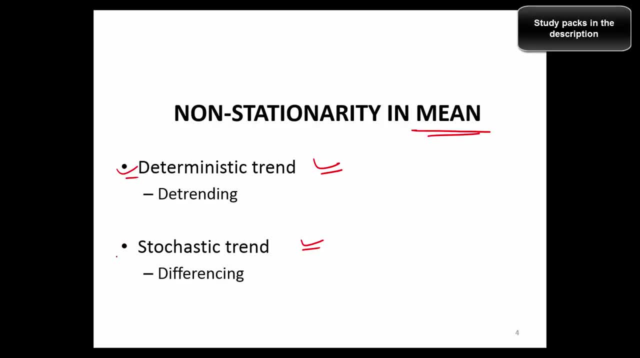 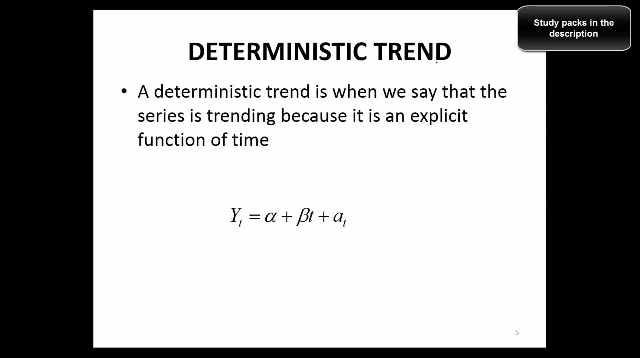 easier to understand and sort of handle, and stochastic trend, on the other hand, is somewhat more difficult because it's uncertain. So let's see what deterministic trend is. So a deterministic trend is when we say that the series is trending because it is an explicit function of time. So that's the definition of a deterministic trend And here's the example. 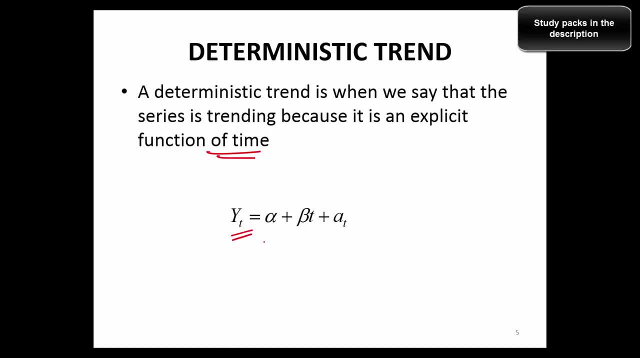 It's simple to understand You. the time series yt is just a function of the time. okay, So yt is just a function of time and nothing else. okay, It's just constant. I mean alpha is just constant. At is this error term? Sometimes, you know, we use that epsilon t. I've just used that at. 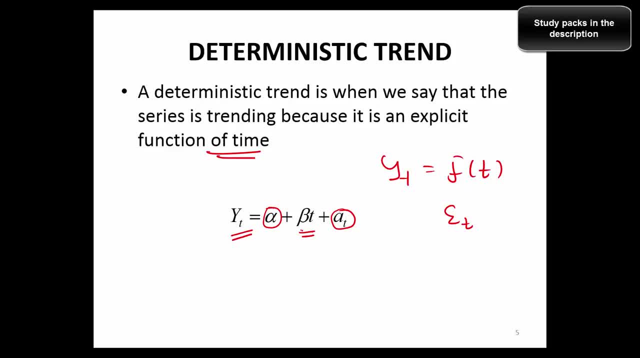 okay, And beta is the slow parameter- okay. So the only variable here in this equation is t, So yt. the time series is a function of time, So it all depends only on the time. So if you increase the time, the value of the time series will go up. So time is not t is a certain variable. 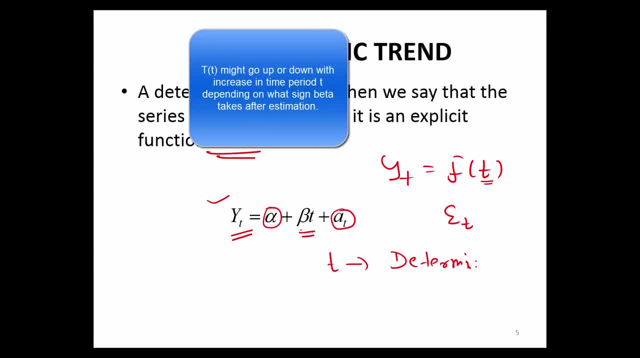 like a deterministic variable, Deterministic or something that is known to us right? So it's not uncertain, so to say, okay, So that's the reason why we call this as a deterministic trend. That means that there is a trend. It's an upward trend. 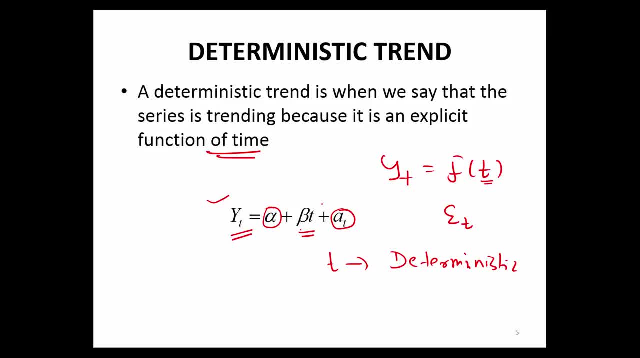 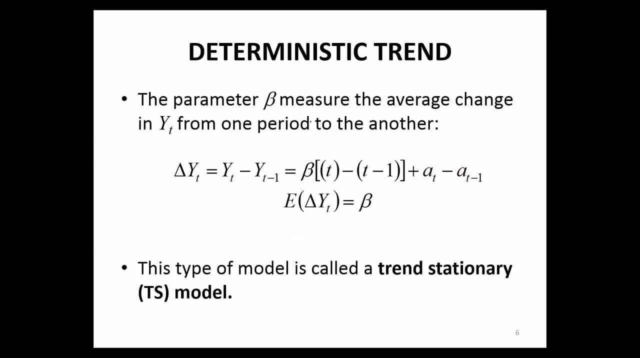 And it is very well known to us because we know what time is. And if you know time, you can very well calculate or find out what the value of yt is. So we'll just try to you know, modify this equation, refresh this equation in a certain way. 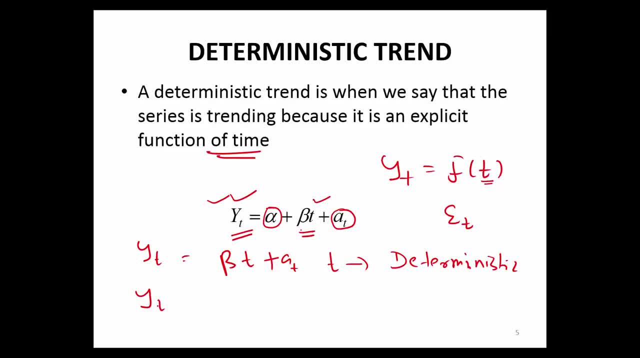 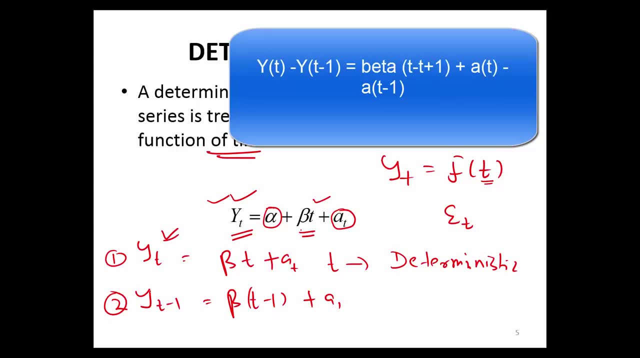 beta t plus at, and then yt minus 1 equal to beta t minus 1 plus at, And then you subtract: this is equation 1,, this is equation 2.. So that means it is the time series equation for time t and this is time series equation for. 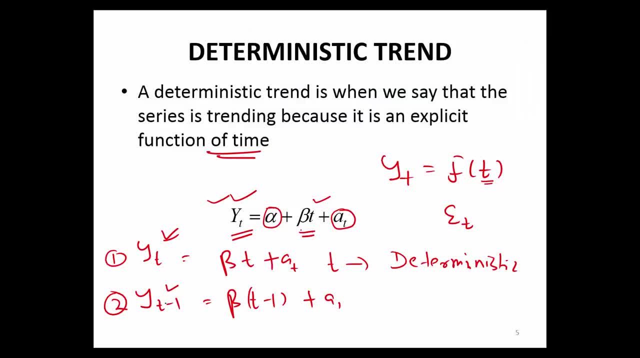 time: t minus 1.. And if you subtract, you know, 2nd from the first, you'll get an interesting pattern. so negative, right? Okay, So here it will be negative. this is positive, So t and t will cancel and what we have is just a beta. okay, That's exactly what we have done here. 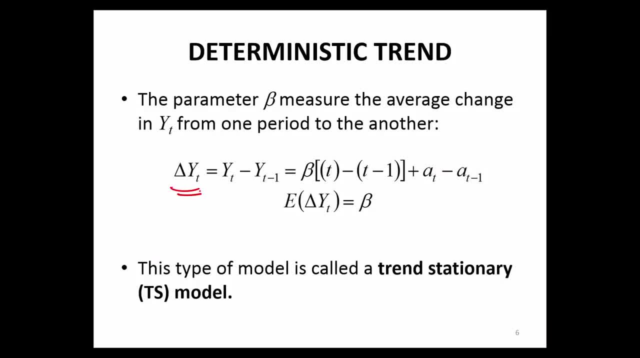 okay, So what we have done here is that this is delta t, delta yt, which is the difference between t minus y, t minus 1. okay, and you know, this is nothing but beta, and you have a t and a t minus 1. okay, and when you take an expectation, expectation of error term, so expectation of expectation is: 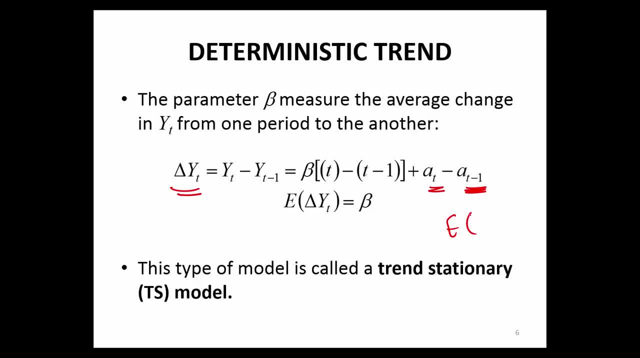 nothing but the mean. and mean of the error term, as you know, is just the 0. the error term is a white noise series and you take the mean of that. it is always going to be 0, okay. so that pack gets cancelled. when you take expectation, so expectation of the change in y t is nothing but your beta and 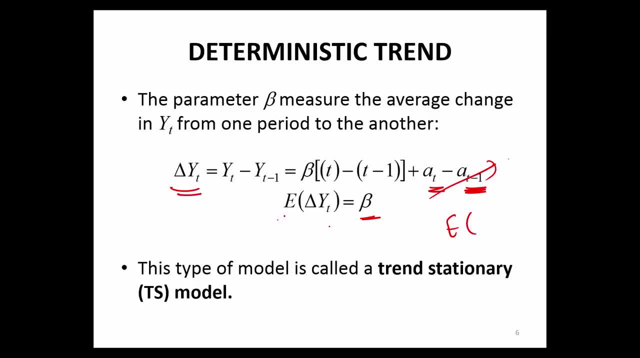 that's the important thing. so in a deterministic trend you take the mean value of the change in your time series. you end up getting what is known as the slope coefficients. so in such a case your slope coefficients is nothing but the difference between the values of the time series for a 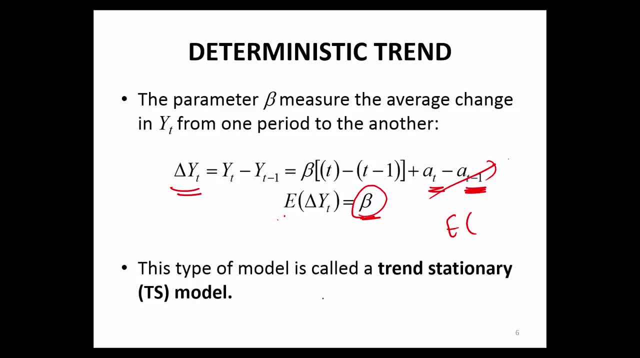 consecutive time period. okay, and that's the reason why this type of model is known as train stationary time series model. okay, that means it's non-stationary but with train. so you can. if you handle the trained, you know you can. you can very well forecast the series without an issue. 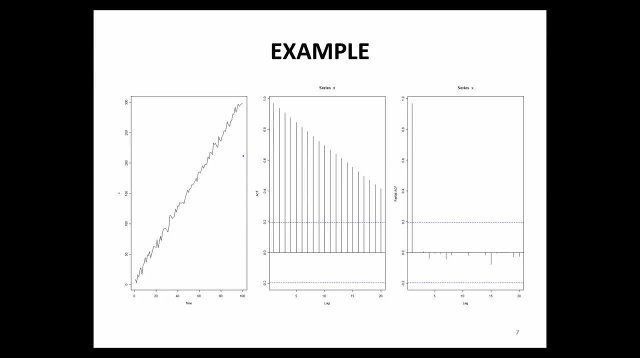 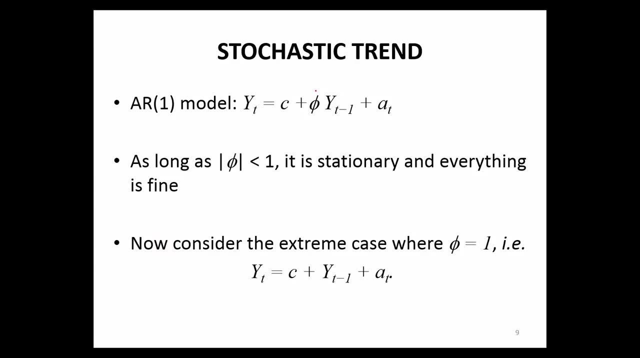 so here is this example. i mean, we have just, you know, simulated some data for it and you can see it is increasing over time with slight variation, and this variation is only because of the error term a, t, okay, and from deterministic trend. so we'll understand how stochastic trend is. 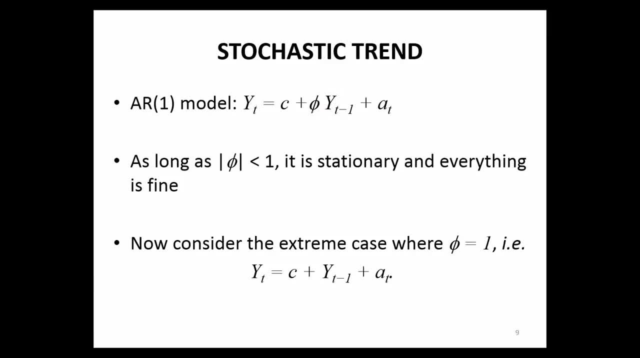 is in fact different from a deterministic trend and how this can be handled differently than the deterministic uh trend. so we'll uh start with an ar type model. so we have y? t, which is a uh, which is just equations. it's like that we have a constant and then it's a function of its previous values: y? t. 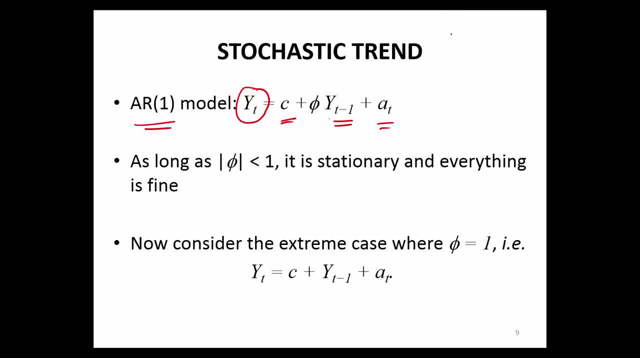 minus one and we have error term. remember in deterministic trend we had y t is a function of just a time. here y t is a function of its past values, y t minus one. so y t can be found out from the previous value of the same time series. now, the previous value of same time series is not. 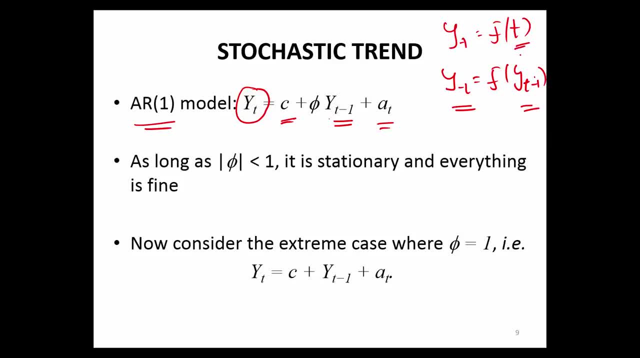 something that is known to us, unlike in the first case, in the deterministic case, where we know for sure what the value of t is going to be okay, and that's why it is called stochastic, because it is so uncertain as long as the phi these slope parameters. so in the in the deterministic case, we 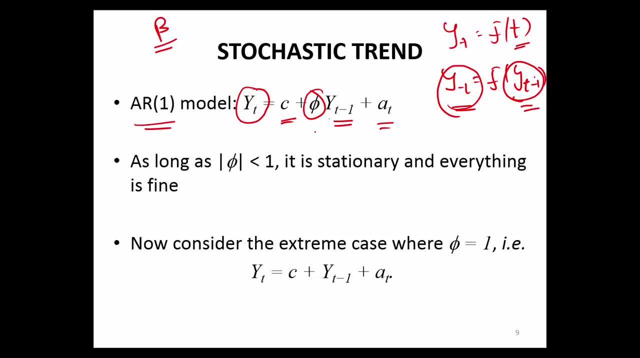 have this beta, right, something similar here. okay, we have used this phi operator. okay, if phi- the modulus of phi- is less than one, then it is stationary and we have no issue with that. you know, we can simply go and do that, and then we can do that, and then we can do that, and then we can. 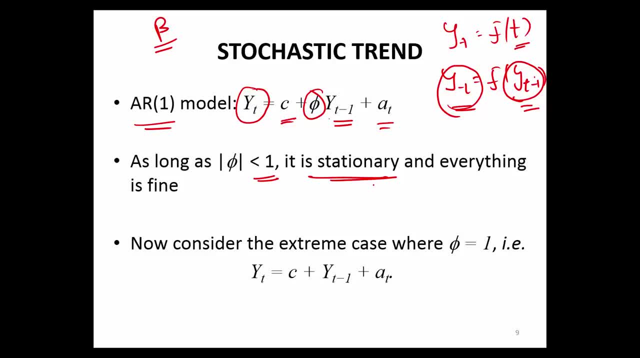 go ahead with forecasting the future values and everything is fine. but there could be cases where this- the modulus of phi- could be the one, or modulus of phi is greater than one. now our topic will- i mean this particular session will- be more concerned about the cases where we have phi equal. 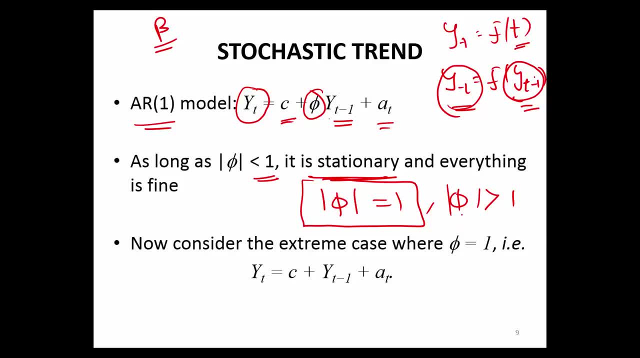 to one. so how do we deal with such case, how do we define this and what exactly is the situation when you have the modulus of phi is is one okay and that's very interesting- um aspect of a stochastic strain which is not that straightforward. it's not stationary, it is. it's a non-stationary case and it's a case that is of 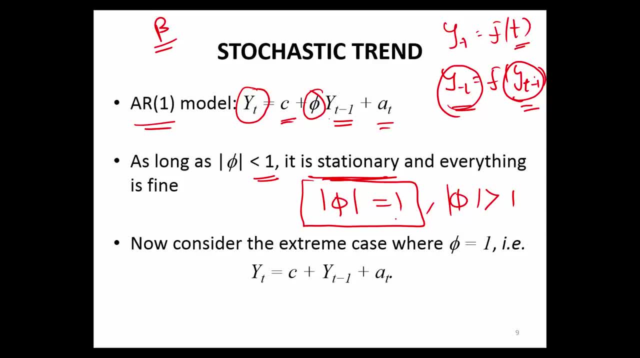 interest to many people, because in the real world, many situations are cases where we have a phi, the modulus of phi, equal to one. in fact, this is some form of random work that we'll be talking about and we'll see in the next few slides. you know what? what the? 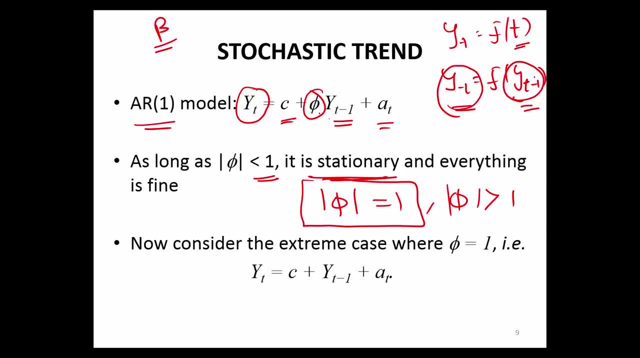 forms are all right. so when takes phi takes a value of one, the series becomes yt equal to constant, and then you have yt minus one, so phi takes a value of one. so there is no coefficient, and then you have the error term right. so if you think intuitively, so uh, let's say you know. 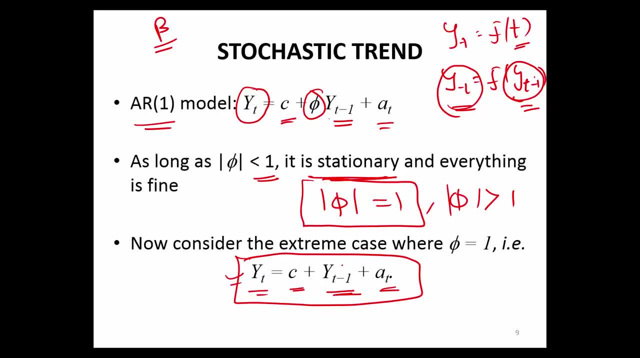 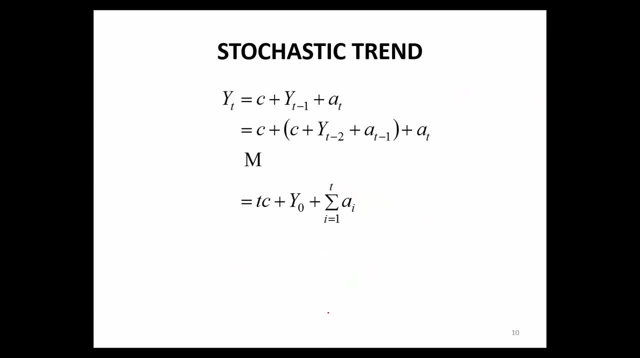 example of stock price. stock price of tomorrow is just the stock price of yesterday plus some constant, okay, and then you have error term, right. such a series is very difficult to focus. this is a typical case of non-stationary series, and we'll talk more about it. so here is this stochastic print where the phi takes a value of. 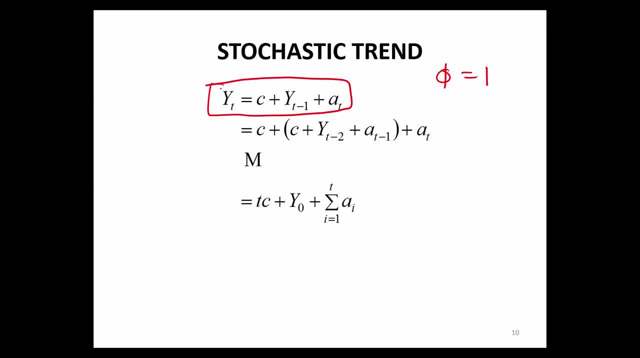 one. so the first series is yt equal to c plus yt minus one plus 80. similarly you can write y, let's say y, t minus one, equal to c plus yt minus two plus a t minus 1, and you put that in this equation. So in place of y, t minus 1, we just put this. 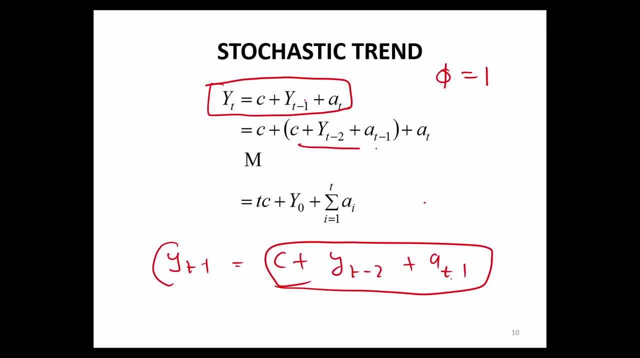 particular equation, and that is what we have done here: C plus this particular thing I have just taken from here. and then you have the error term, And you keep doing that for y- t minus 2, you can also write that in terms of y- t minus 3, and you keep doing that and ultimately you will. 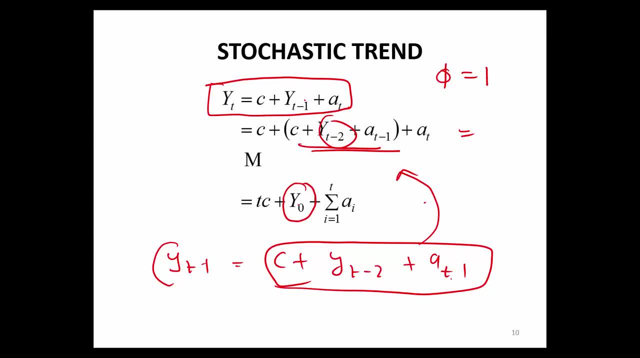 reach a point where you will have y 0. And you have t times the constant and you have summation of the error terms which eventually, you know, gets to. So why do we really want phi to be less than 1? for you know stationarity and so on. So what happens when phi is less than 1 is that: 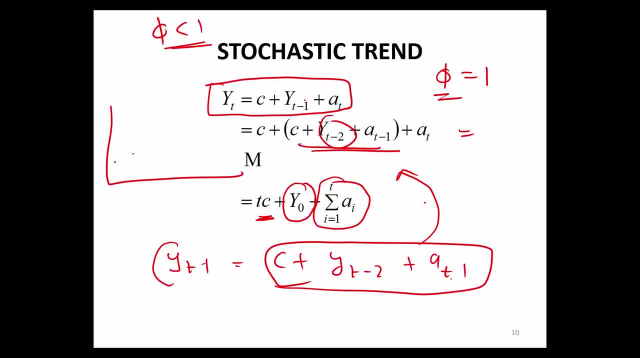 when you plot the time series. it is going to be mean reverting. That means the time series will come back towards mean every time it goes up. If it goes up, it is going to be mean reverting. So that means it is going to be mean reverting. 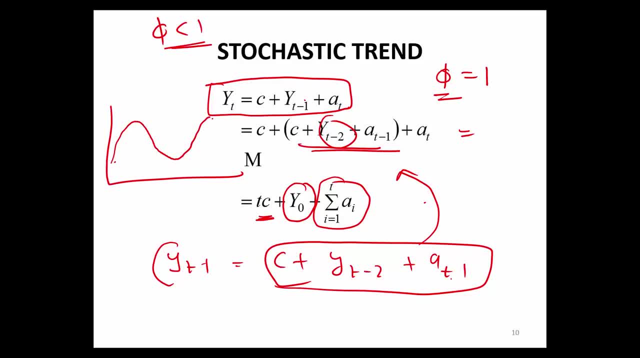 It will certainly come towards here, and then it goes up and comes towards, So it will be somewhere near that mean. So the mean will be constant and, moreover, the variance will also likely to be very- you know- constant or near constant. So that is one of the property of 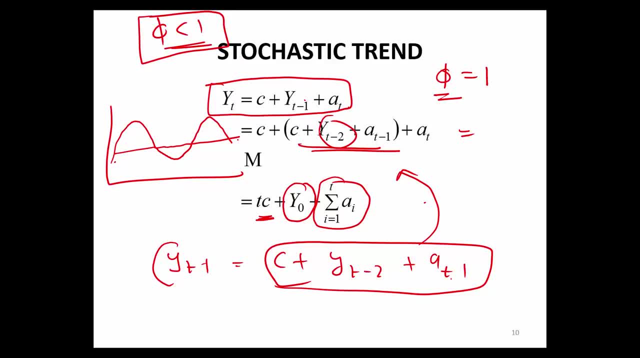 phi being minus 1. here You can actually mathematically prove that the series is converging if phi takes a value of, you know, less than 1. Otherwise it is not going to converge. So this is a typical case of a random work model. So y t equal to y t. 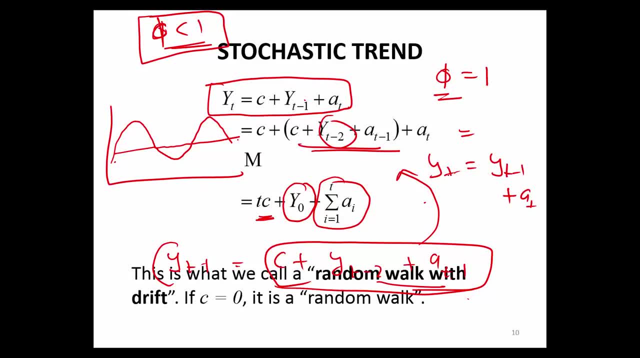 minus 1 plus the error term a, t. So this particular thing is a typical case of random work, And if we include the constant part, then it is dripped. That means the series has started not just from 0 origin. It started somewhere here or somewhere here. 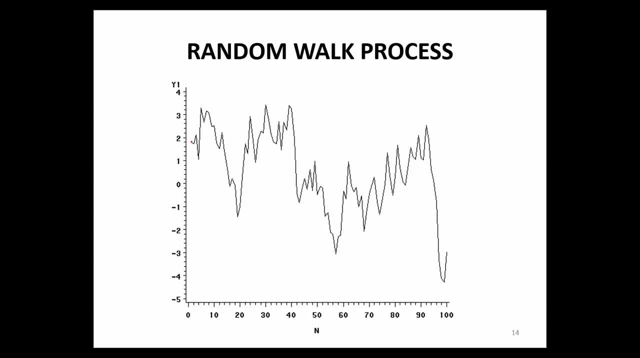 Some negative or positive values Looks something like this. It looks very weird. There is no trend at all, There is no pattern. So basically, what random work means is that there is no pattern in the data. There is no pattern in the data, Just you know, pure random, And there is nothing in. 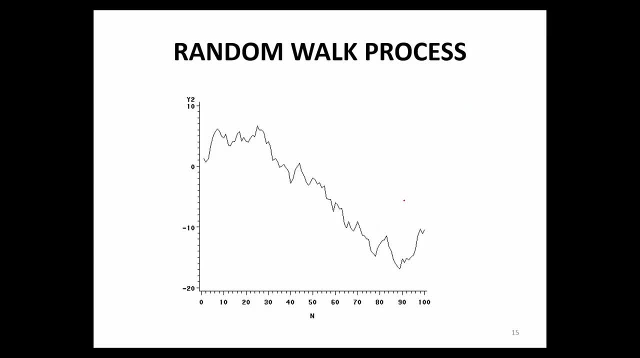 the data that you can use for forecasting your future- Something similar. So this is also a typical random work process. So random work process can be closely related to the behavior of stock market. Stock market also many a times does not have much of information in the past values, Although many people will say. 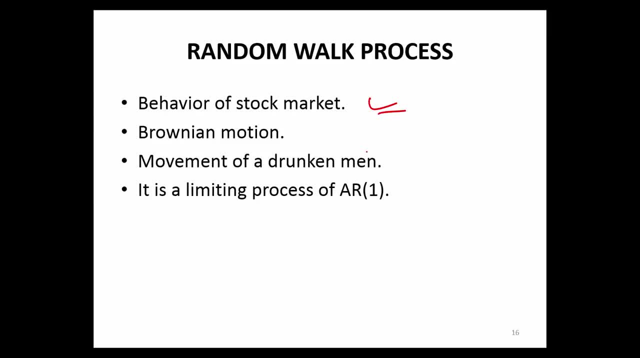 that forecasting stocks, price or return is very much possible. But that is not always always the thing. Stock market many times behaves purely as a random work. Sometimes it has some pattern, but many times it has no pattern in it. It's also used in in understanding. 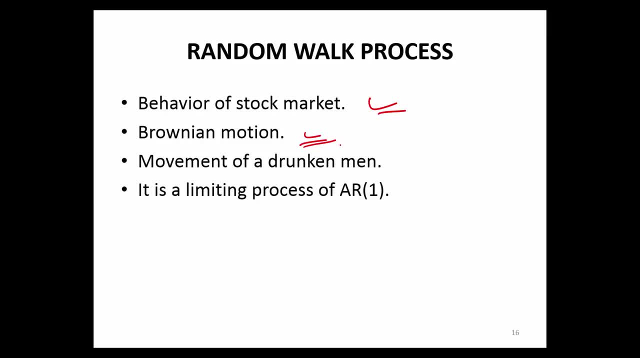 Brownian motion. in many science and science areas, also in finance, A movement of a drunken man, somebody with a drunk, you will have no pattern if you and if you try to understand or study his pattern of walking, there's no pattern at all. So it's also a limiting process of an 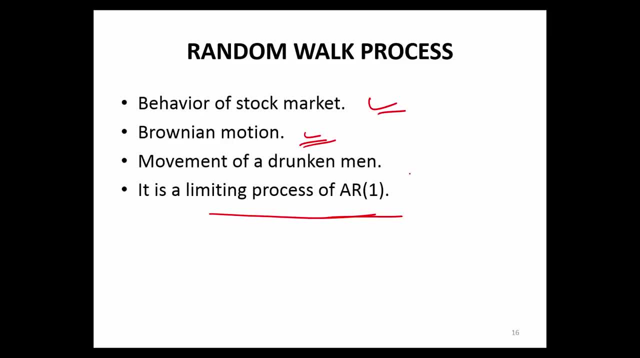 Ar1 process. So Ar1 process is just yt equal to y, sorry, yt equal to phi, y minus T plus A T, Right? so this is an AR1 process. so when phi equal to 1, you take the random process. If phi is less than 1, you have the AR1 one. So this is: 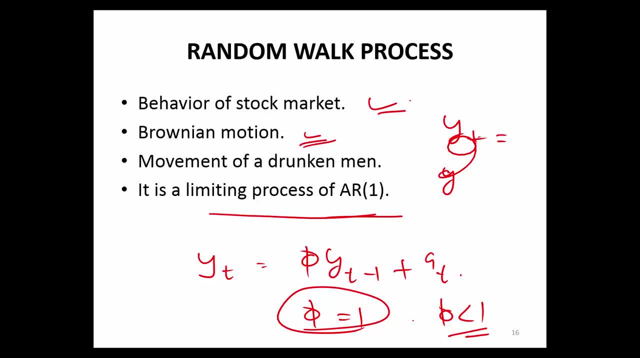 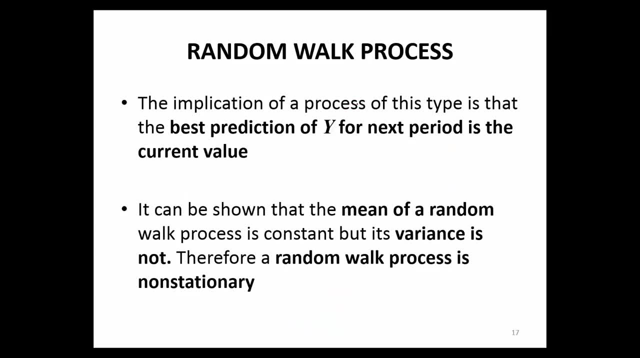 typical condition for Ar1.. So random walk is basically the special case of Ar1 where I should say random walk. so random walk is our traditional, where you cannot go ahead in building a forecasting model. So what the implication, what is the understanding or the takeaway point? 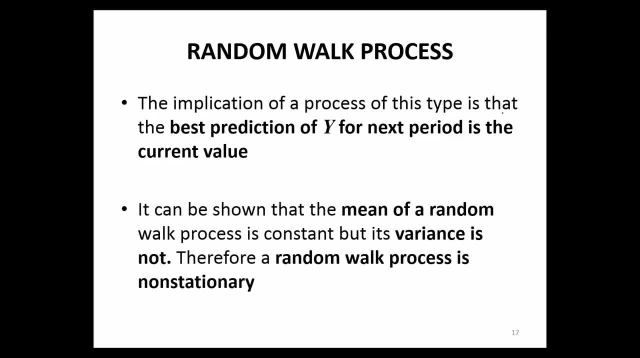 The takeaway point here is that the implication of process of this type is that the best prediction of y for next period is the current value. Now, if you have a time series data and that follows random work, just stop there, do not have to do anything, So you all need to. 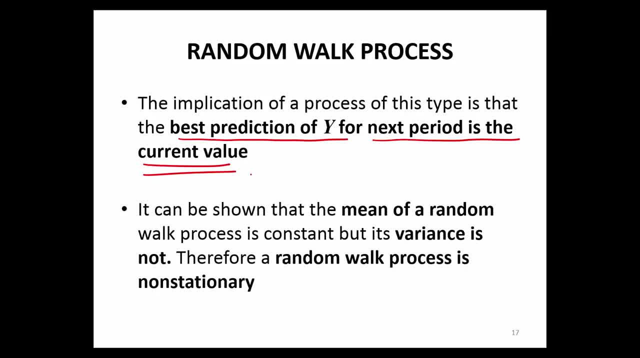 convey or you need to communicate to the audience, is that the best prediction for this particular time series, for future is nothing but the current value. There is nothing that can. nothing more can be done, other than that It can be shown that the mean of a random 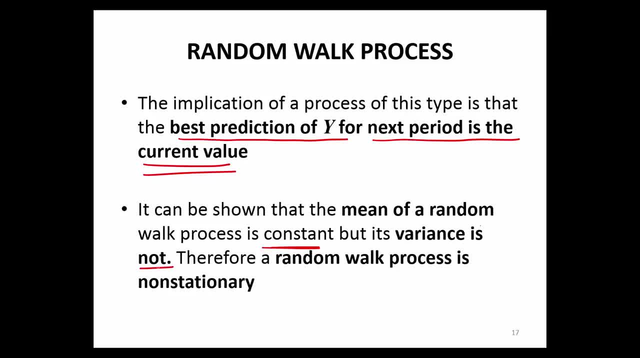 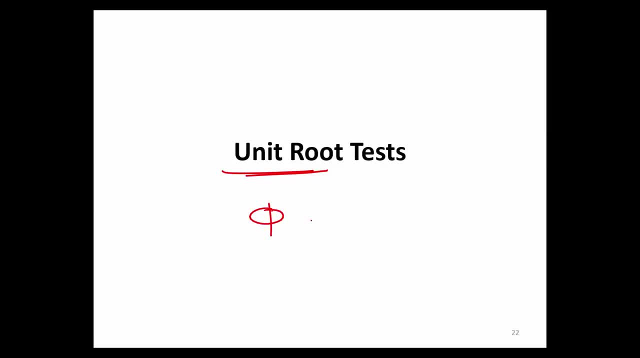 work process is constant, but the variance is not Okay. So the name, such as unit root, means we are only talking about how to find out whether the phi that we talked about in the non-stationary series is 1 or not. Okay, So, in a stochastic, 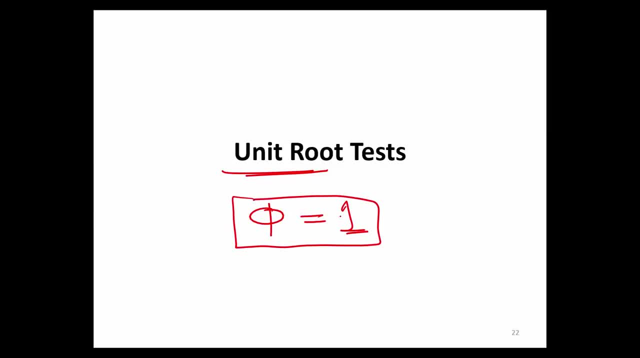 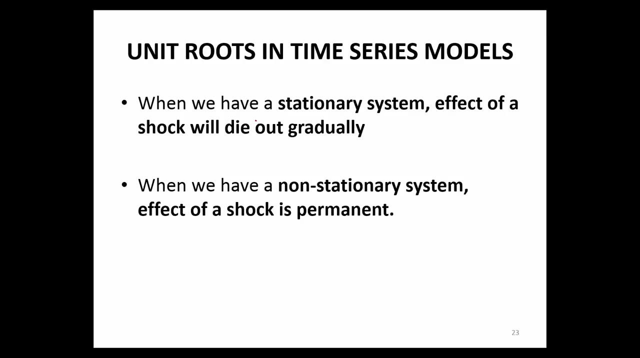 train series that we have just learned. if phi is 1, then we are sure it is the random work process and that is what we call as unit root, and we need to statistically test that before getting to know. Okay, So when we have a stationary system, 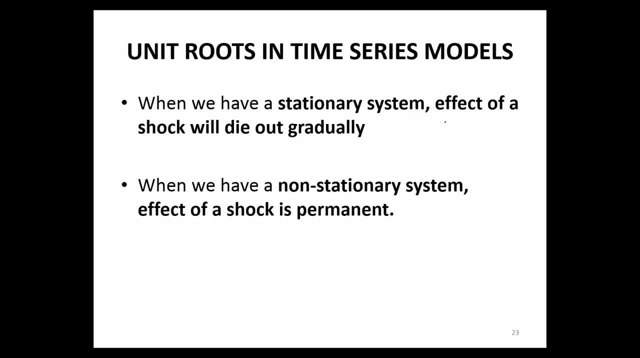 we know for sure that the effect of any shock that is going to happen to the time series will die out gradually. Okay, In a stationary series, if you have a shock, it moves up, it eventually comes down and then it removes somewhere in the mean. and then, even if 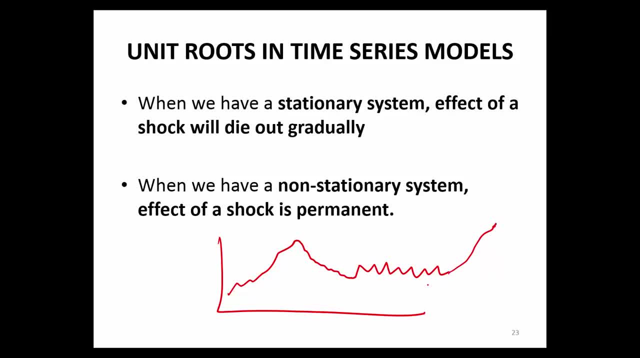 another. there is a shock in upward or whether it is downward it is. if there is downward shock here, it will again come back. But that is not the case in non-stationary system. In non-stationary system, if there is a shock, okay. if, if, if something goes up. 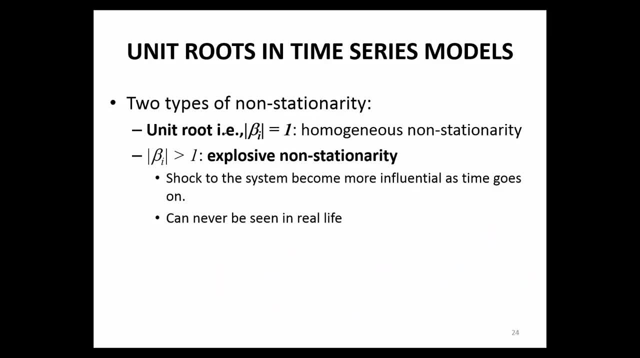 it never comes down to the mean. All right. So there are two types of non-stationary. Okay, One case where you have the, you know this case is just 1 and the other case is phi is greater than 1.. We have we just taken beta, just keep changing notations, But 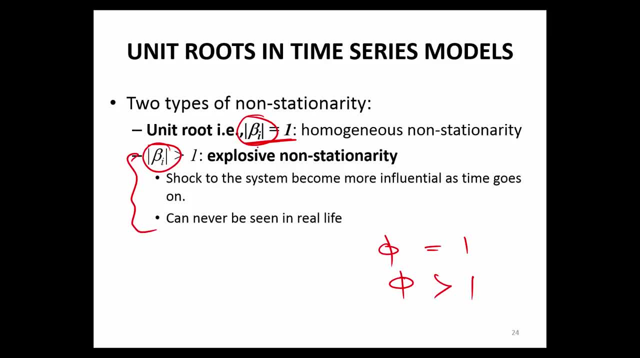 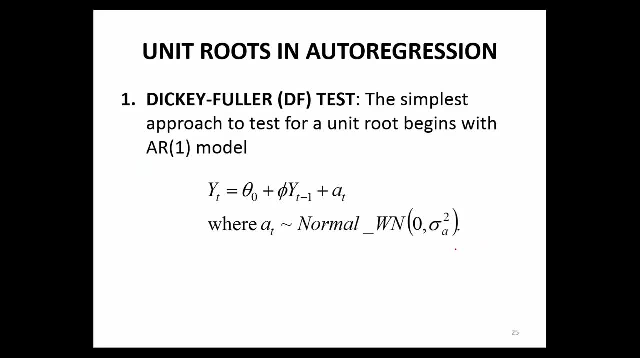 you know, the second case we, of course, will ignore for here. So the first case we would like to see when is the case when we have the phi equal to 1 and that we can get to know using Dickey-Puller test? Okay, 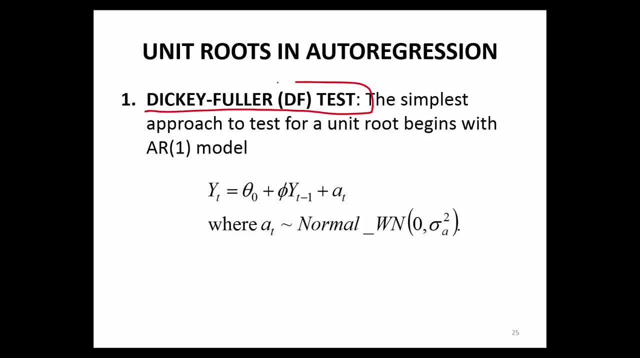 So this is a test using which we can find out whether there is presence of unit root or the time series is unit root or not. So unit root is just- you know another way of saying that- whether it is a random work series or not. all right, So the simplest approach is just to have a 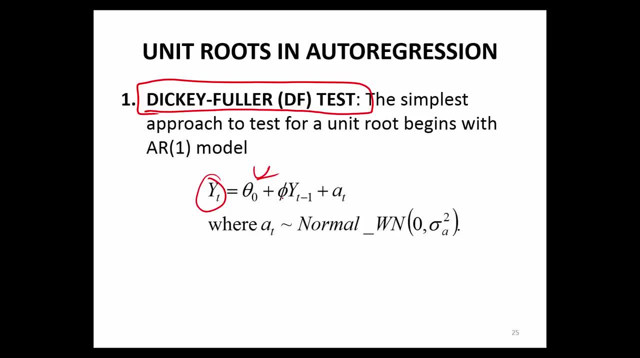 air 1 series, yt with the theta and we have psi of yt minus 1, and we would like to know if psi is sorry, if phi is 1 or not. Now, this is air 1 series, right, and we expect phi to be less. 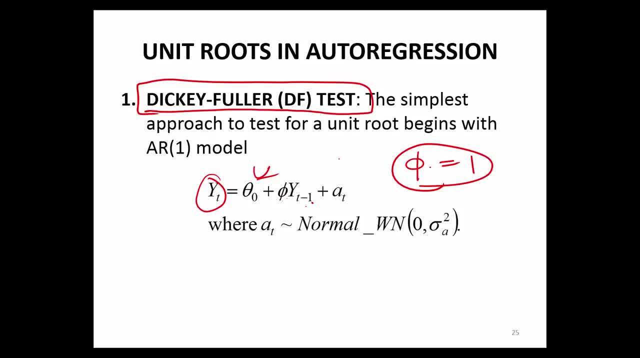 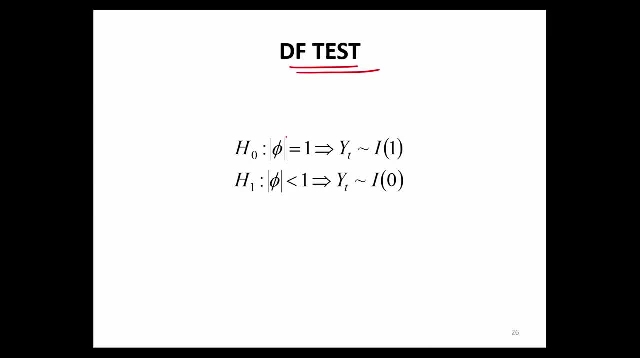 than 1.. If it is equal to 1,, then that is a problem. that is a random work series, right? The hypothesis testing in the case of a dicupulus test is like this: the modulus of phi is either 1 or modulus of phi is less than 1, which is the alternative hypothesis. 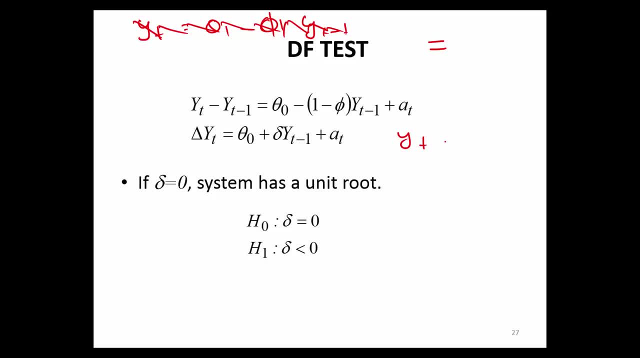 So we have the series yt equal to yt minus 1, this is theta, not plus at. and then what do we do is that we simply subtract yt minus 1.. So, from left and both right, yt minus 1.. minus yt minus 1 equal to theta naught. sorry, phi, sorry, this is theta. sorry, theta naught. 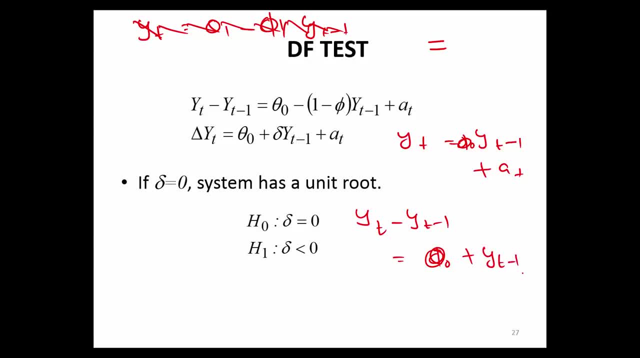 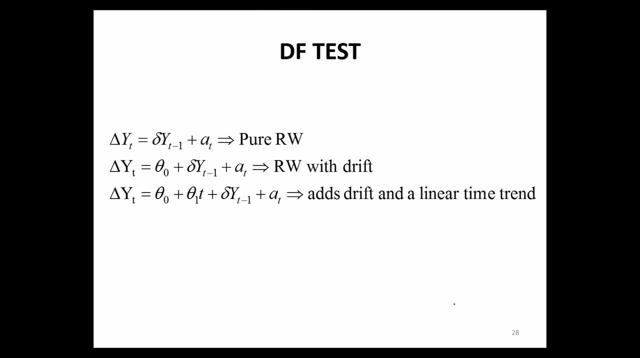 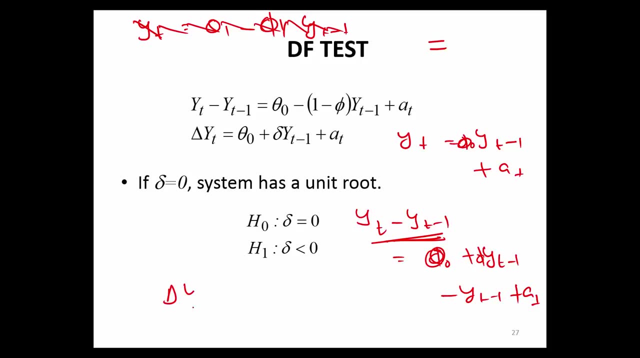 plus yt minus 1, which is again psi phi here minus yt minus 1 plus. at Now this is just delta d, So delta yt is equal to theta naught plus. here we can take yt out, So yt then inside we. 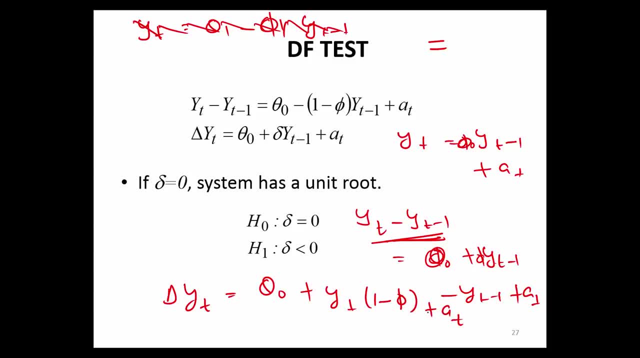 have 1 minus phi plus at, And then 1 minus phi we just denote with some other symbol So this particular term. if it is equal to 0, then we have unit rule, otherwise not. So it has now changed. So null hypothesis is now: either it is 0 or it is less than 0. 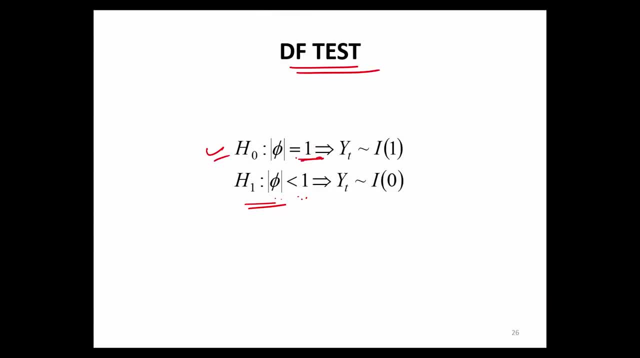 So just slight change. here we are comparing with 1 or less than 1, here it is: either it is 0 or less than 0.. There are three types of Dicke-Fuller test we can do. I am not going to the details of 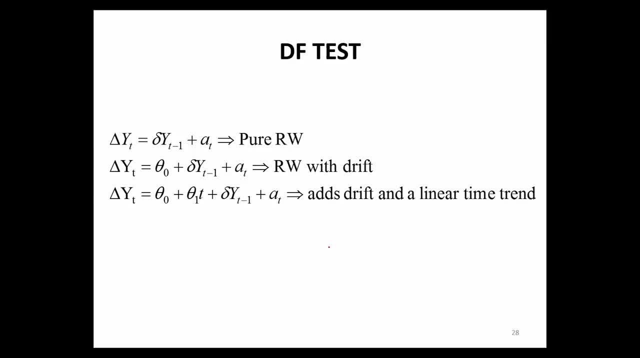 it. but depending on the kind of random work we are trying to understand, we will have different type of Dicke-Fuller test. The first case is a pure random work. There is no drift, There is no theta term here, It is just. 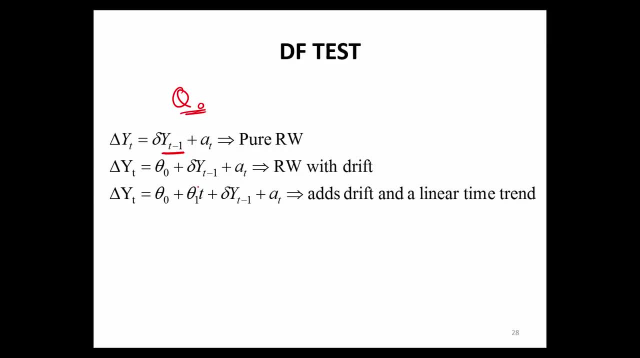 the past value of yt. So we would like to know if the coefficient is 0 or not in this case. The second case, we have a drift And in the third case we have a drift And we also have a deterministic time component. We have theta 1t, So time it is the deterministic time. So we have a time component, So we have theta 1t, So time it is the deterministic time, So we have theta 1t, So we have theta yt, So time it is theta 1t. Sove is just the combination of the. 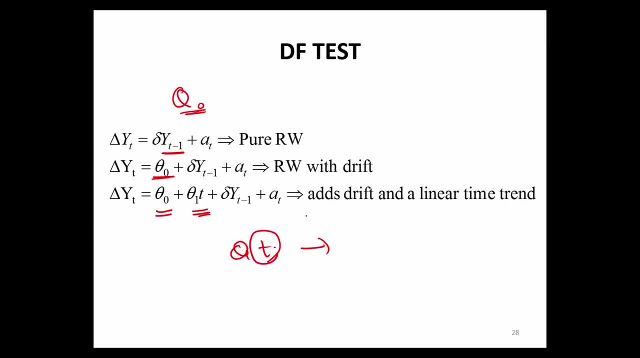 deterministic and stochastic time. Leave your time trend So that three types of Dicke-Fuller test we can do, depending on what type of what the intention is. We can also do all three and see which one is actually is the best for the given time series data. So how do we find a? 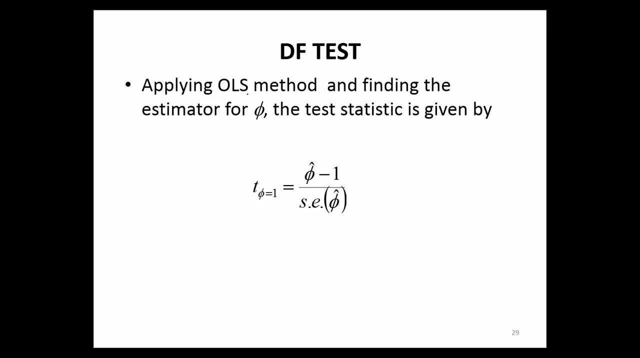 test statistic. here You just apply OLS, you know, you have the equation, Regression equation. so we we just find, we just estimate the parameters. So parameters: here is phi, remember, is 1 minus phi. we just change it to different symbol. but ultimately we are trying to find out what phi is. 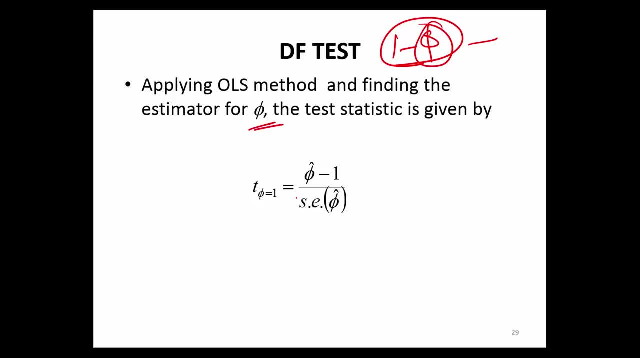 So we can find that out using OLS, and then we can find out the t statistics. we can find out the t statistics and then we see whether it is significant or not. the methods would not allow you to, let us say, in a forecast future. you rather take more of a guess, depending. 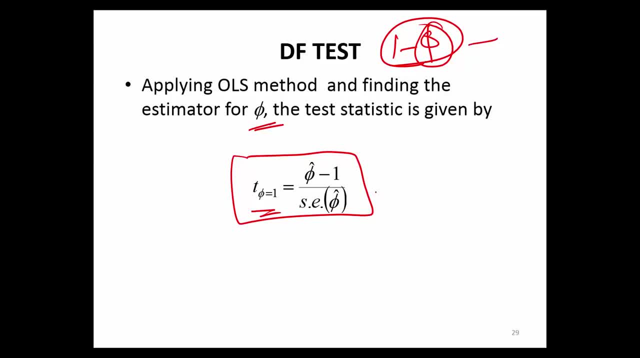 on the past values of the time series, rather than doing some sort of analysis that is not going to give any accurate. So that is one of the important test that people do before we even starting to explore other time series models for forecasting, and it is quite